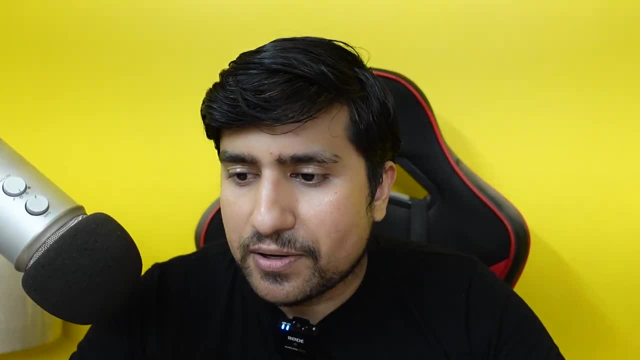 you can see if you know what you should know. So let's get started and let me explain you how you should know the concepts or not, alright, So let's get started. So, guys, it's a very big one, but I will try to explain it. See how big it is because it contains lots of details, but we will. 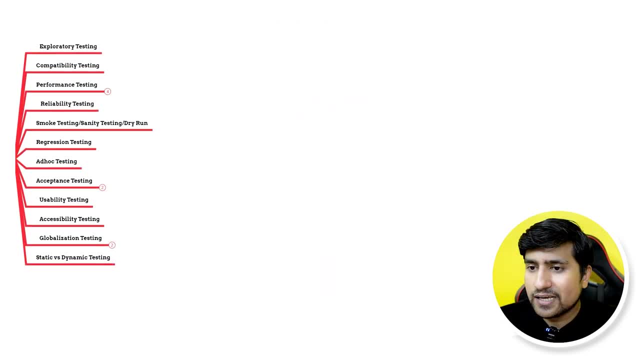 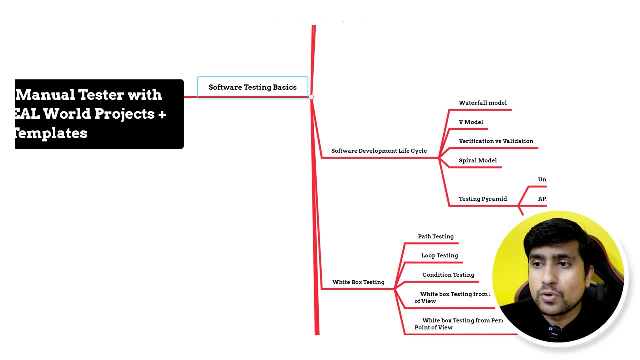 go one by one and we will go with the different things. that, what exactly are the things that you should know? First of all, you need to pay attention to the software testing basics. okay, In the basics, what you should know. you should know about the different type of softwares. What? 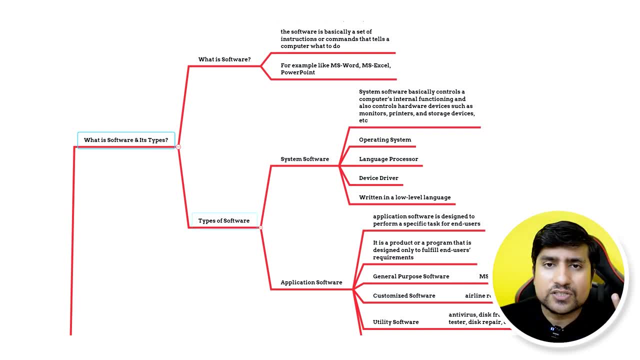 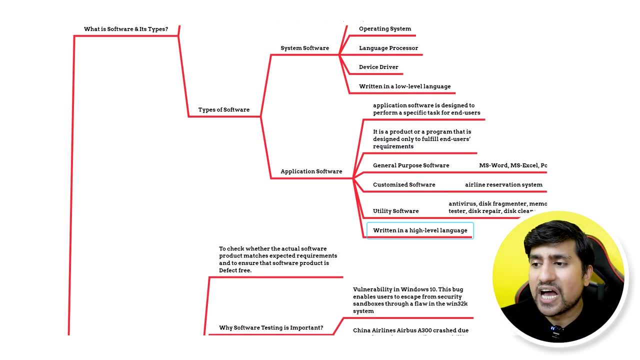 exactly is a software? Different types of softwares are available, right, We have system software, we have application software, we have general purpose customized utilities and high-level language written softwares. I have explained them with a proper example. You can go through it. After that you have to focus on the software testing You have. 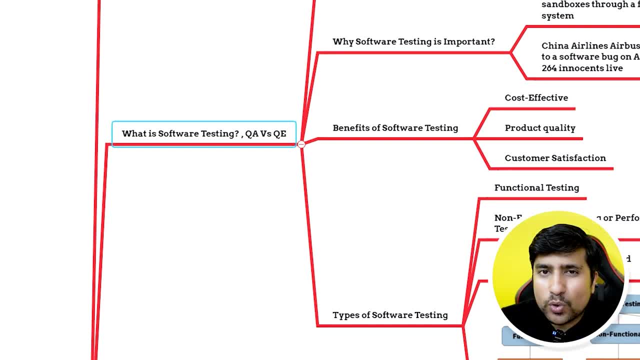 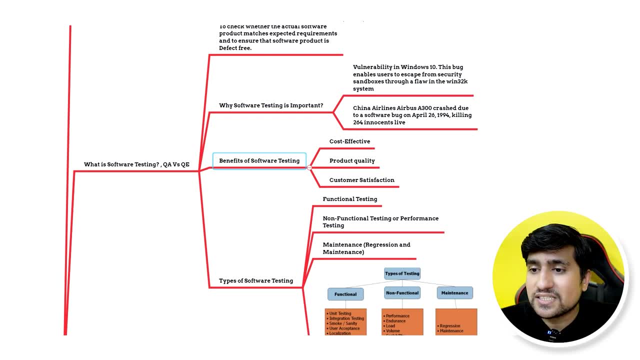 to focus on what exactly is a QA QE. Sometimes people call it QA QE, software tester, manual tester. What exactly these different things are there? right, You have to know about the different benefits as well as the types of the software testing that you should have. So we have a. 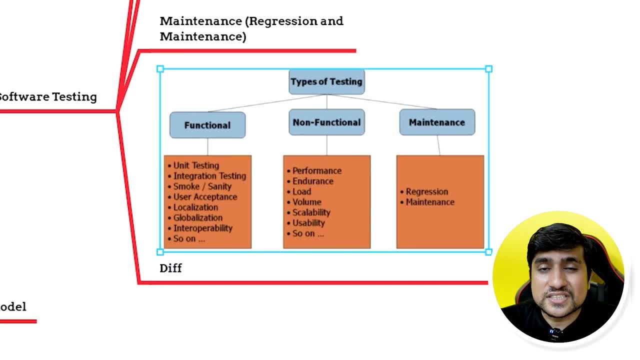 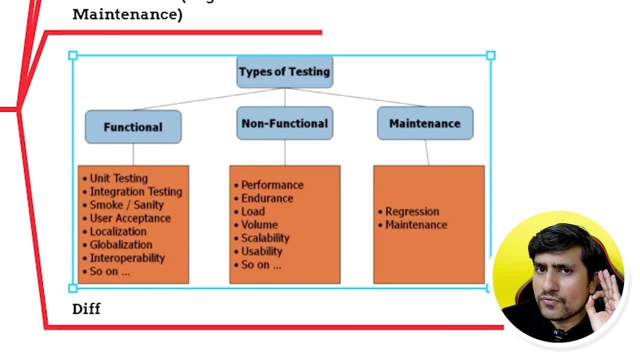 functional testing, non-functional testing and the maintenance right. So in the functional testing, different type of testing related to unit testing, integration, smoke and all the things you should know. In the non-functional one also, you should know few of them. For example, 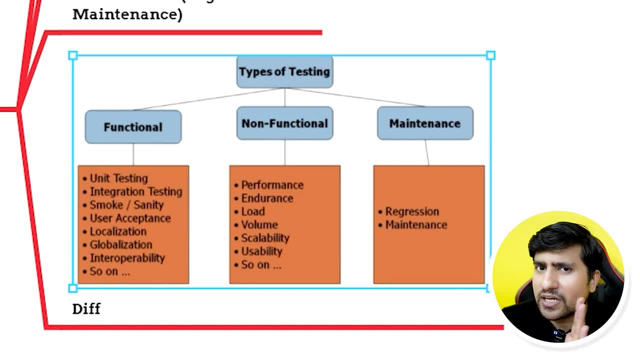 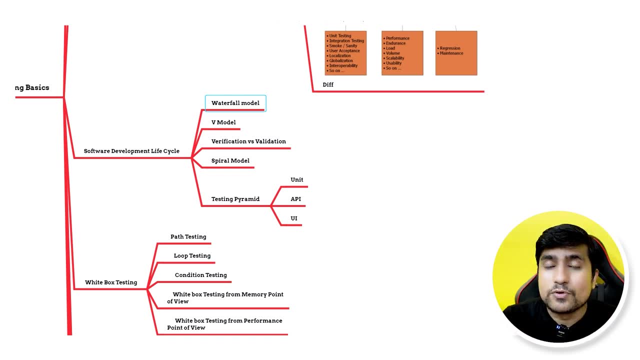 performance, security, usability, acceptance- other things that, as a non-functional, you should focus on. it Now comes to the very important thing, which is software development lifecycle. Many times in interview, people ask questions related to waterfall and V model, So you can learn more. 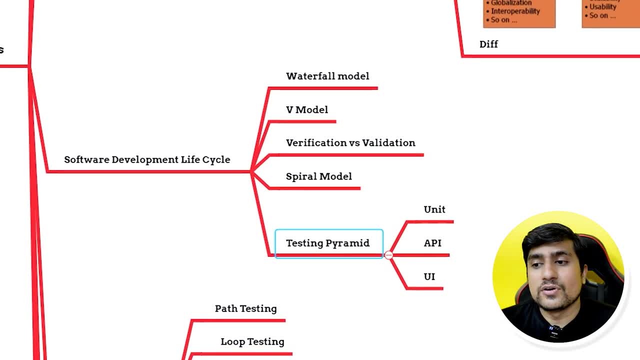 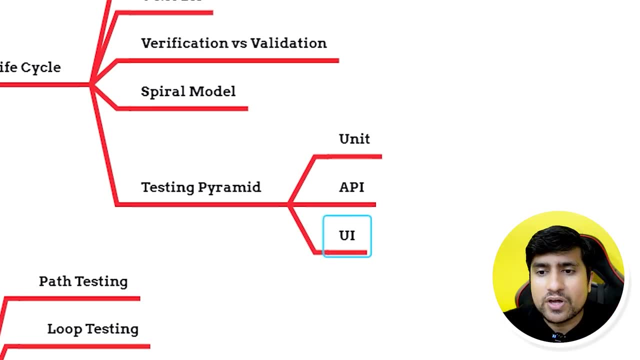 about it. I would highly recommend you to pay attention to the testing pyramid, where you will learn about the unit testing, API testing, as well as the UI testing which, basically, most of the time, you will be doing in a functional manner. okay, Again, as a software developer, you should. 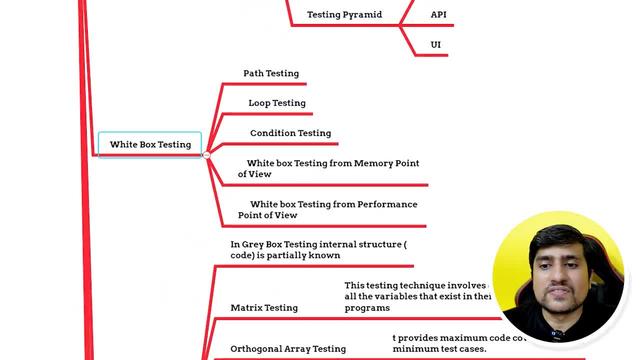 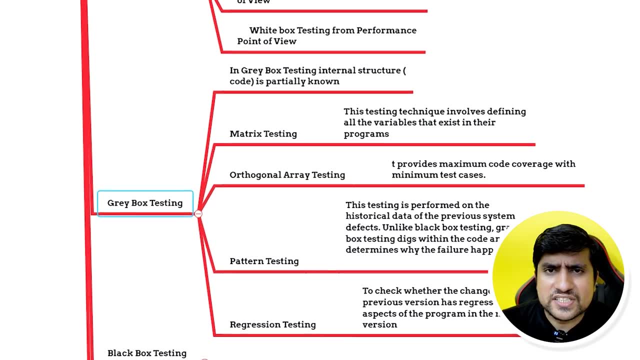 know the different things related to the UI box, For example part testing, loop, conditional and other things, and all Similarly in the grid box of testing. it is a type of testing, guys, where we have to know the different techniques available. Again, for black box, we already know we have. 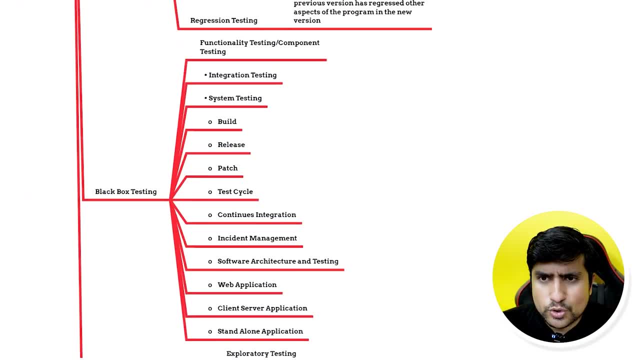 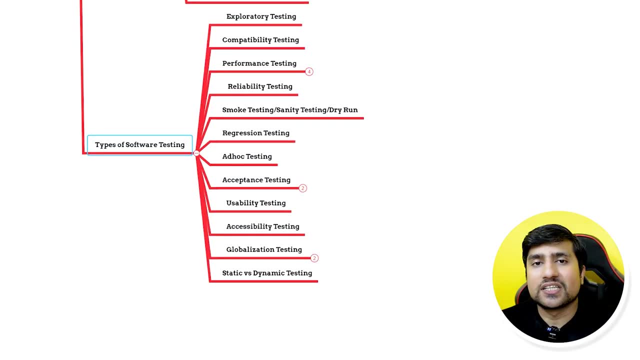 different type of to design the test cases. we have many, many things that we should know: integration system testing, continuous integration, client server and different things related to it right. Similarly, we have more software testing type like exploratory. 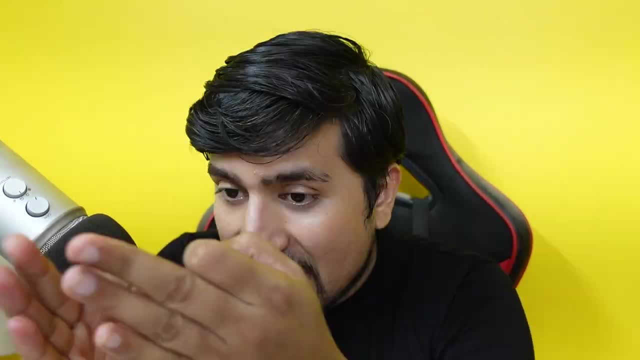 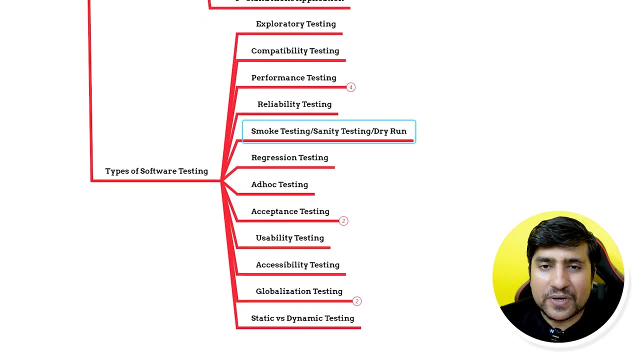 compatibility, performance, reliability and other things. Again, as a software developer, you should know some of the definitions and probably some of the work that you have done right, Like exploratory performance, reliability, acceptance, usability- many times throughout your career. 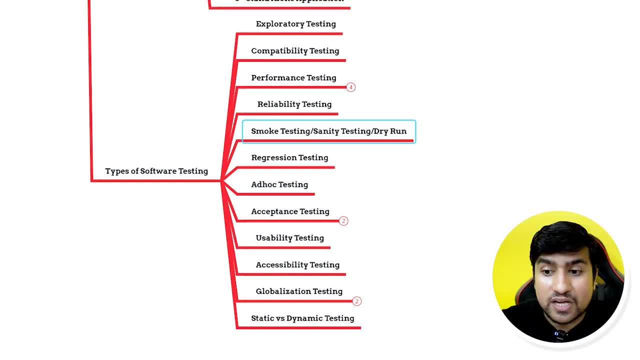 right. With my 10 years experience, I think I have done many, many different types, For example globalization. I have done usability acceptance, I have done ad hoc, I have done exploratory, I have done performance, I have done reliability testing, I have done smoke testing. So, yes, 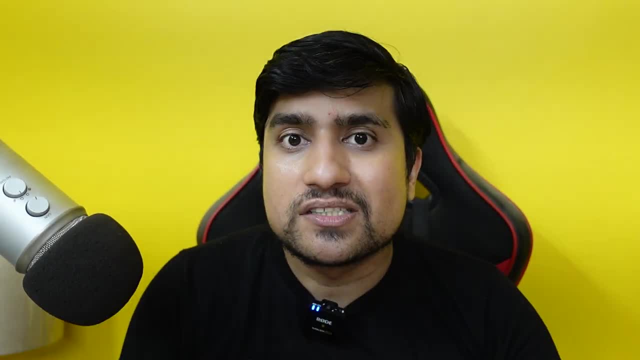 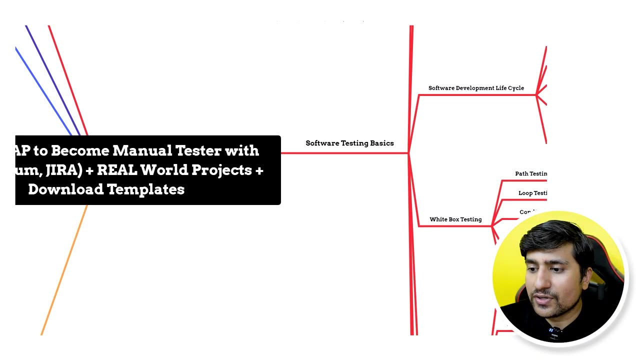 throughout your career you will learn about it. So, as a fresher or even as a manual tester, focus initially right These topics. you should do that, okay. So now I think the basics are clear. So whenever you are clear with the basic, 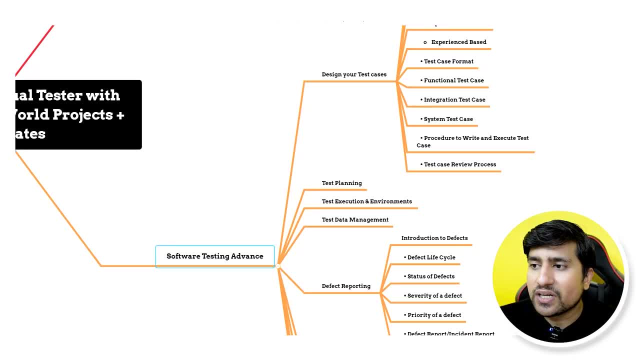 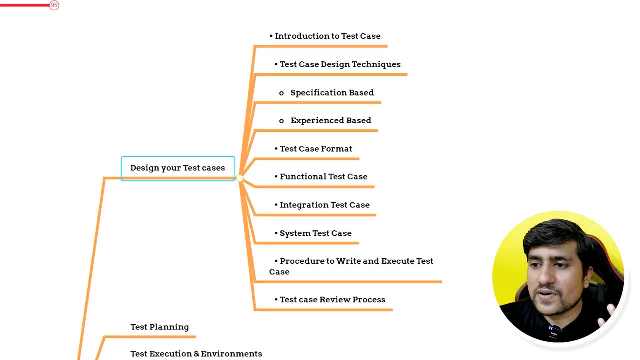 you have to jump to the advanced. We are in the advanced. we are going with the test design techniques right. You should know what exactly is a test case, test scenario, test format. how to write your functional test cases right. Different procedure: test planning. 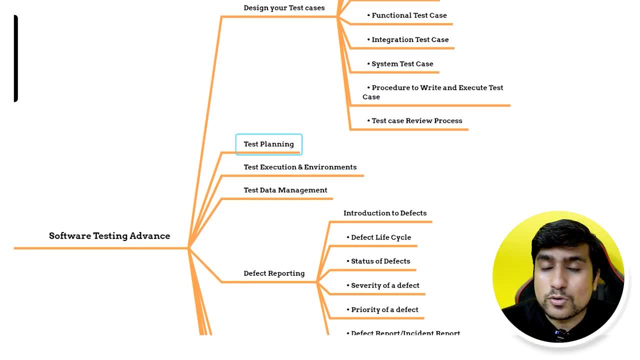 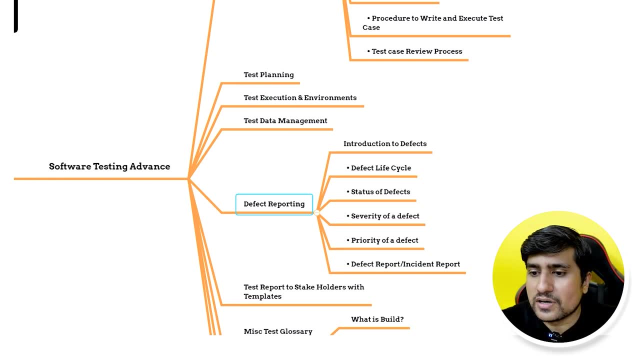 because test planning is really, really important, guys, I have put a template also- you can download the template- the antif's environment defect reporting, which is a really, really important skill for you guys to learn Test management tools like Practitus. 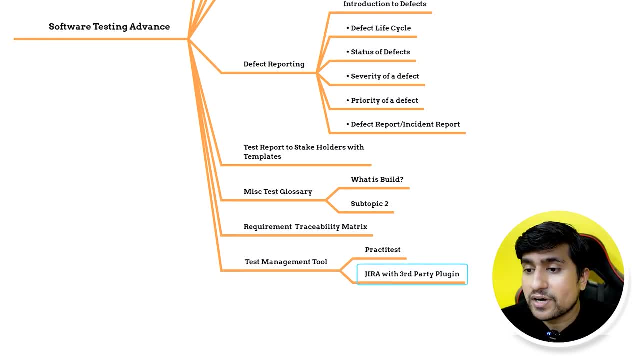 Zephyr Zira with third-party plugins- right, You should know about it. pay attention to that. RTM, as well as the RCA root cause analysis. you should know about it. So these are the advanced concepts related to the software testing that I have put. Pay attention to that, okay. 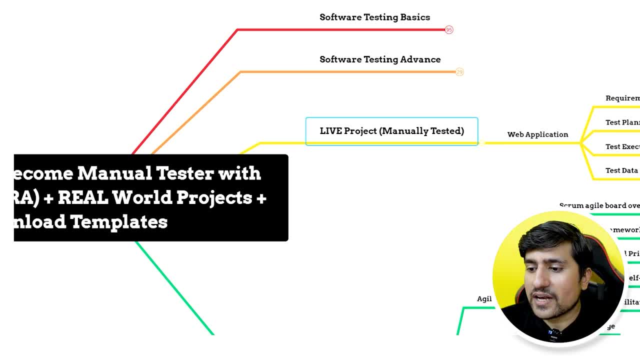 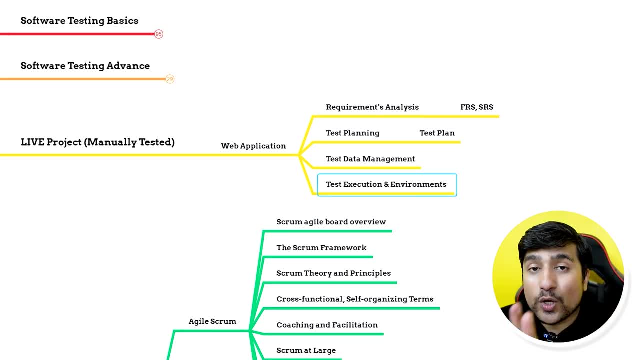 Now let's come to the important topic, which is live projects. Again, I have added a couple of projects where you can take some web application from the requirement till the execution right. You have to know the end-to-end STLC lifecycle right, So that's where we will learn more about. it Again. now it is the end-to-end STLC lifecycle, right, So that's where we will learn more about it Again. now it is the end-to-end STLC lifecycle, right, So that's where we will learn more about it. 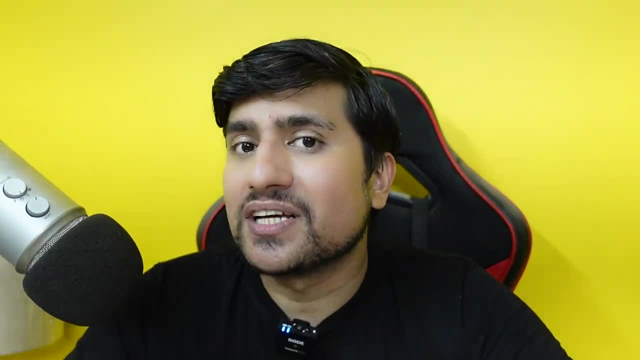 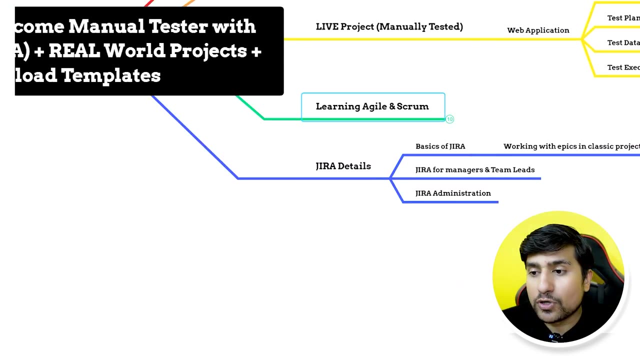 It is mandatory for all of us to know, to learn about the Agile as well as the Scrum. So, yes, in the Scrum concepts that you should know and Agile Kanban also you should know. So those things I have added in the roadmap also, Again, really, really important topic, which is Zira. 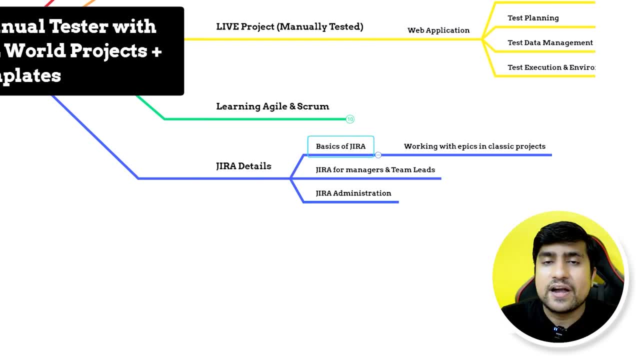 administration, as well as the basics right- How we handle epics, what is the bug lifecycle in the Zira and how different estimations are done. you should know as a manager, as a team lead in the Zira detail. This is really, really important nowadays, okay, So I hope this is.